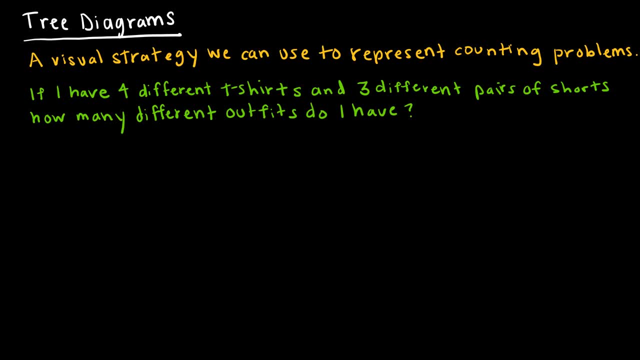 If, instead, you were asked to find what number of outfits you could create with four t-shirts and three different pair of shorts those different outfits were, then we might use a strategy called a tree diagram, And a tree diagram is just a visual representation. It's going to help us see what those outcomes are Now. 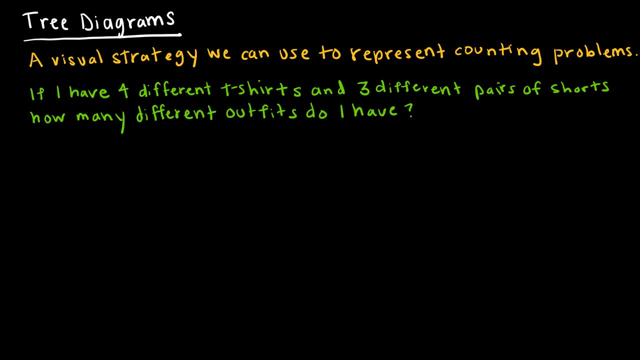 tree diagrams are most helpful when you would use the product rule, So when you have different outcomes, that you would multiply to find the number of options, or, once we talk about probability, the probability of those options. But let's get started on this one. Notice I am going to make four branches because 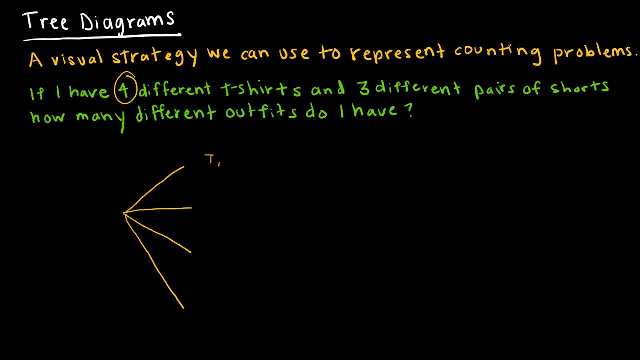 I have four different t-shirts, So I'm just going to call this t-shirt one, t-shirt two, t-shirt three and t-shirt four, And then, off of each of those, I am going to make three branches, because there are three options for the next one, And so here I would write: shorts one, shorts two. 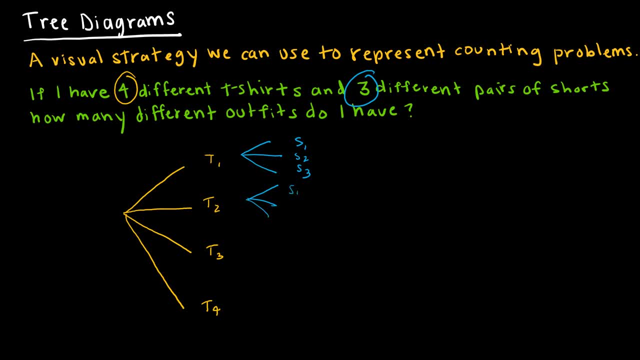 shorts three And I would do that for each of these. And again, it's not super helpful in this question because I gave a sort of an easy question to look at. But the very important last step that a lot of students forget: 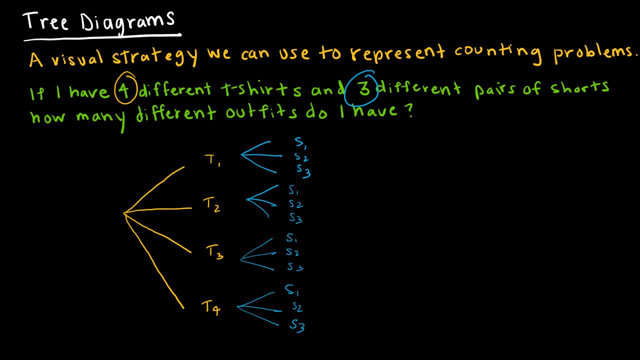 to do is to look at what the total outcomes are. So when I'm writing what the outcome is, essentially I'm following the branch. So I would follow the branch to T1. And then, from there, follow the branch to S1.. So this one is T shirt one, shorts one, And then I 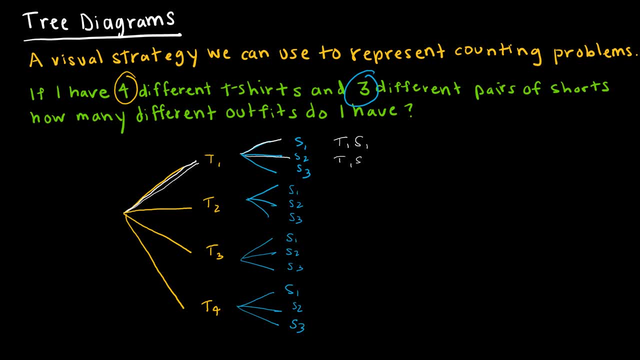 could do T shirt one, shorts two, And T shirt one, shorts three, And I could continue that all the way down the list. Now, what's going to be important here is we have already determined that four times three is 12. And there are 12 different options, And if I were to list all of these, there would 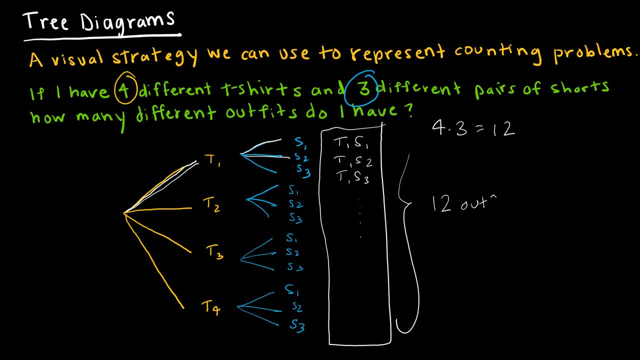 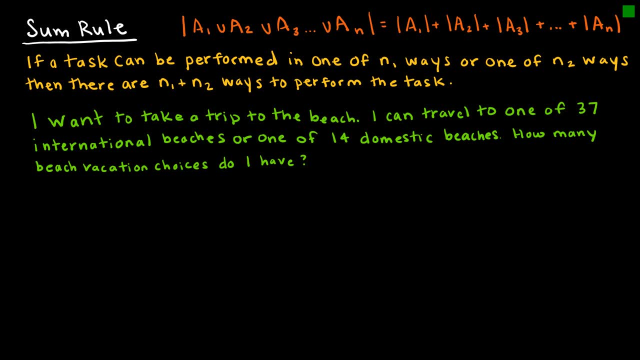 also be 12 different options. So I would have 12 different options And if I were to list all of these, there would also be 12 different outfits that I could wear. The sum rule is if I have a task that can be performed in one of n-1 ways or one of n-2 ways, 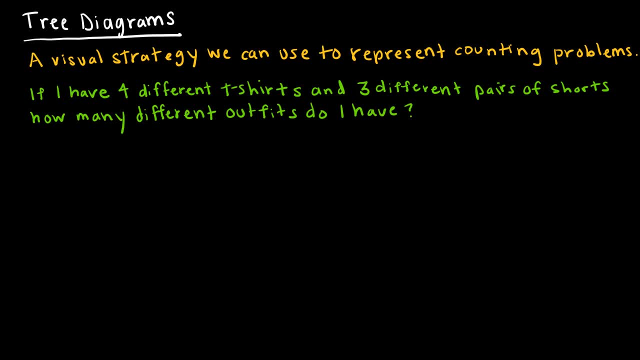 tree diagrams are most helpful when you would use the product rule, So when you have different outcomes, that you would multiply to find the number of options, or, once we talk about probability, the probability of those options. But let's get started on this one. Notice I am going to make four branches because I have 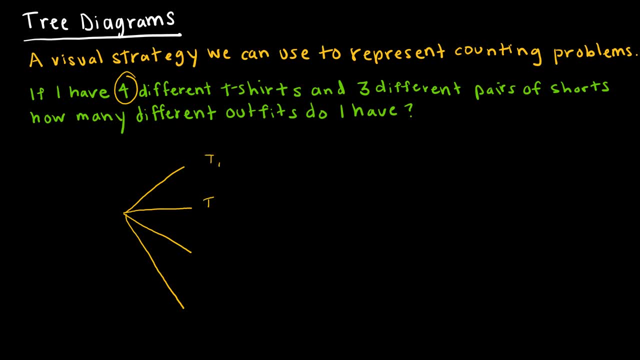 four different t-shirts, So I'm just going to call this t-shirt one, t-shirt two, t-shirt three and t-shirt four, And then, off of each of those, I am going to make three branches, because there are three options for the next one, And so here I would write: shorts one, shorts two, shorts three. 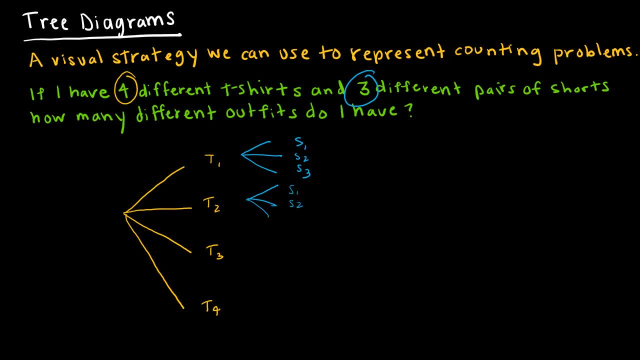 and I would do that for each of these and again, it's not super helpful in this question because I gave us sort of an easy question to look at, but the very important last step that a lot of students forget to do is to look at what the total outcomes are. so when I'm writing what the outcome is essentially 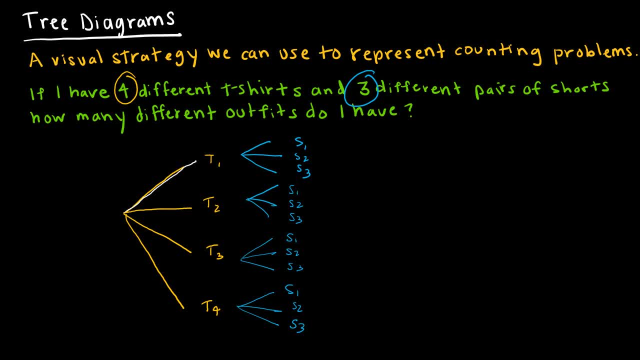 I'm following the branch, so I would follow the branch to t1 and then from there follow the branch to s1. so this one is t-shirt one, shorts one, and then I could do t-shirt one, shorts two, and t-shirt one, shorts three, and I could 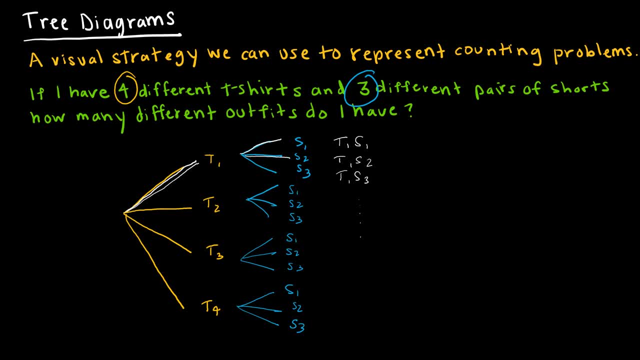 continue that all the way down the list. now, what's going to be important here is: we have already determined that four times three is twelve and there are twelve different options. and if I were to list all of these options? and if I were to list all of these options, and if I were to list all of these? 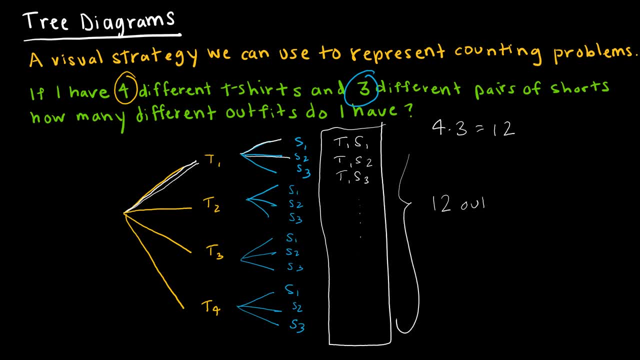 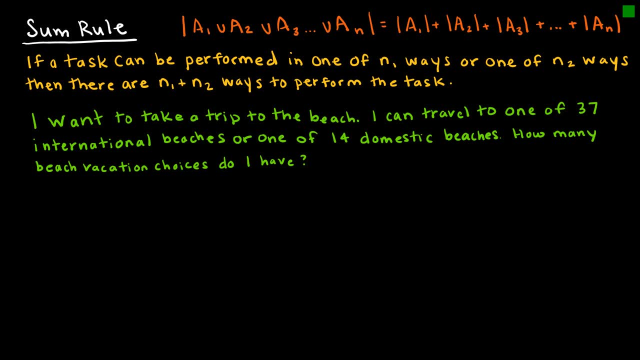 there would also be twelve different outfits that I could wear. the SUM rule is if I have a task that can be performed in one of n one ways or one of n two ways, and so or is our keyword here? with the sum rule, then there are n plus one plus. 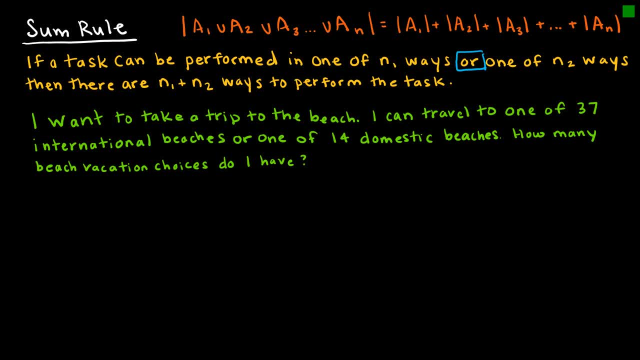 sorry, and one plus n, 2 ways to perform the task. so, for instance, I always, I always want to take a trip to the beach, but let's say I can either travel to one of 37 international beaches or one of 14 domestic beaches- How many? 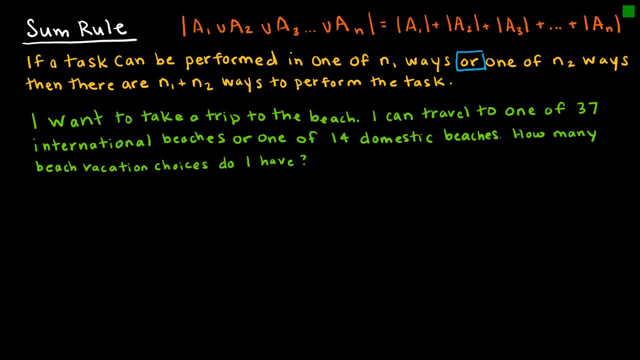 and so- or is our key word here? with the sum rule, then there are n plus one, plus- sorry, n-1 plus n-2 ways to perform the task. So, for instance, I always, always want to take a trip to the beach. But let's say I can either travel to one of 37 international beaches. 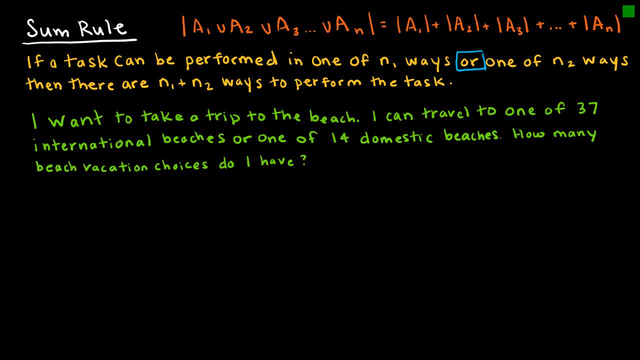 one of 14 domestic beaches. How many beach vacation choices do I have? So all this is saying is, if I can take 37 international or I could take 14 domestic, then there are a total of 51 beach choice vacations that I have Now. 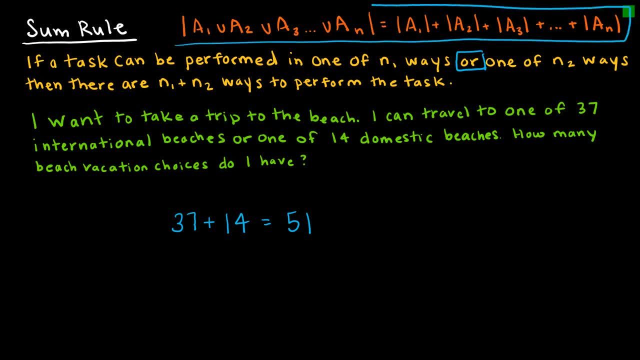 notice. I've written the sum rule out symbolically for you above and that's just saying if I can perform the task. and these lines on the side that looks like absolute value. that's just the cardinality. It's saying how many are inside that union. and so this is saying if I've got some choice of a1 or a. 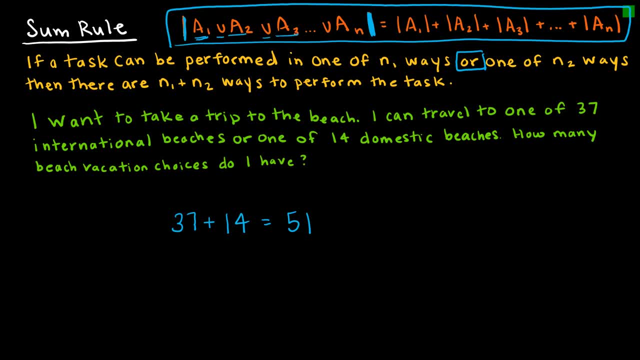 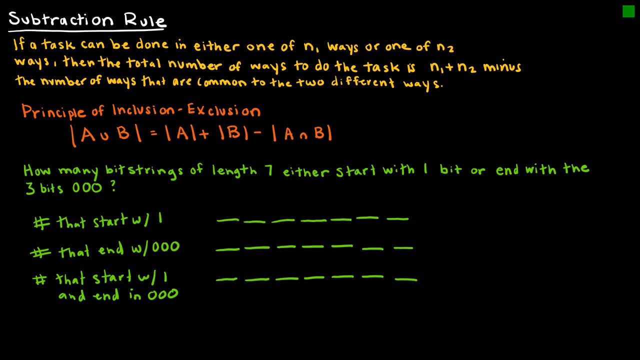 choice of a2 or a choice of an a3, etc. then all I have to do is add the number of each of those choices to find the total number of choices. Now we have the subtraction rule, and quite often you will see this called the principle of inclusion-exclusion, and we'll talk more in. 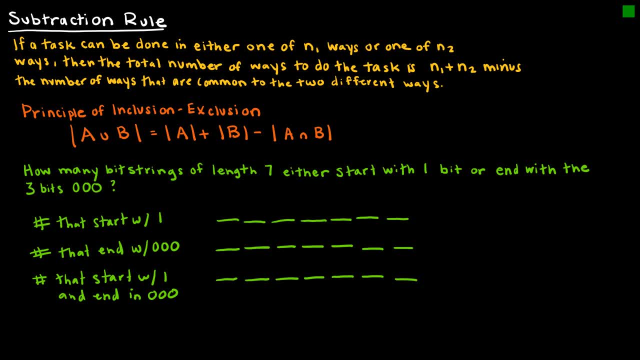 detail in this course and then we'll talk in way more detail if you continue on to combinatorics. But the subtraction rule basically says: if a task can be done in either one of n1 ways or one of n2 ways, then the total number of ways to 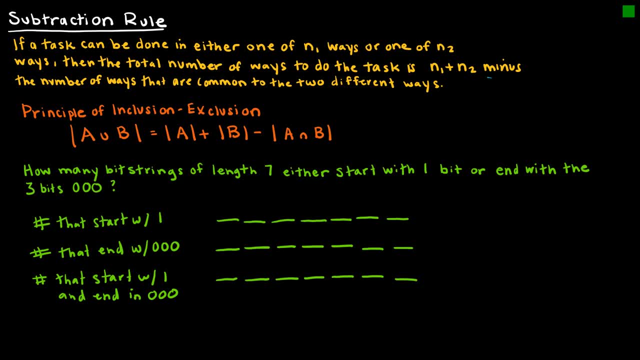 do the task is n1 plus n2 minus the number of ways that are common to the two different ways. So essentially, if you've taken any sort of statistics class, this is the rule that says: hey, if there's something here in the middle where those values are not disjoint, so there is an overlap of the 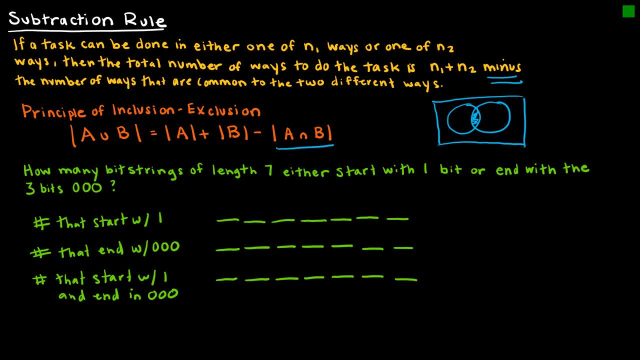 number of ways in each set. then we have to subtract what's in the overlap, because essentially it was counted in the first set and in the second set. So for instance, how many bit strings of length seven either start with one bit or end with three bits? zero, zero, zero. So if I have the number that 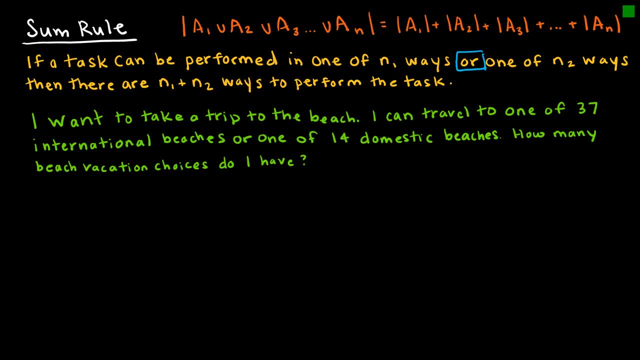 beach vacation choices do I have? So all this is saying is if I can take 37 international or I could take 14 domestic, then there are a total of 51 beach choice vacations that I have Now notice I've written the sum rule out symbolically for you above And that's just saying if I can perform. 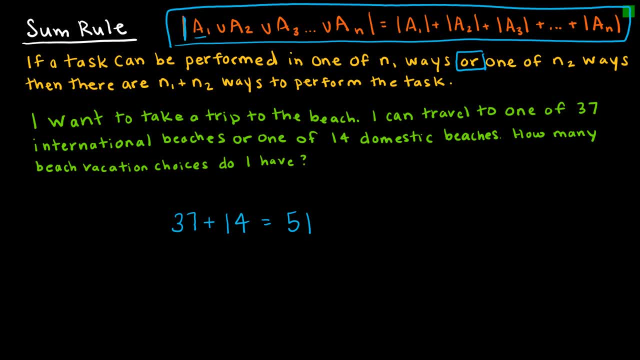 the task and these lines on the side that looks like absolute value. that's just the cardinality. It's saying how many are inside that union And so this is saying: if I've got some choice of A1 or a choice of A2 or a choice in A3, etc. 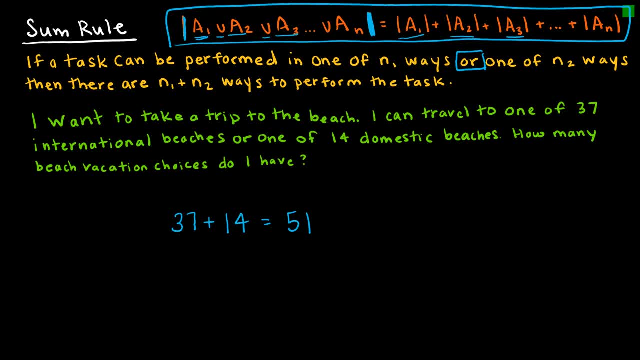 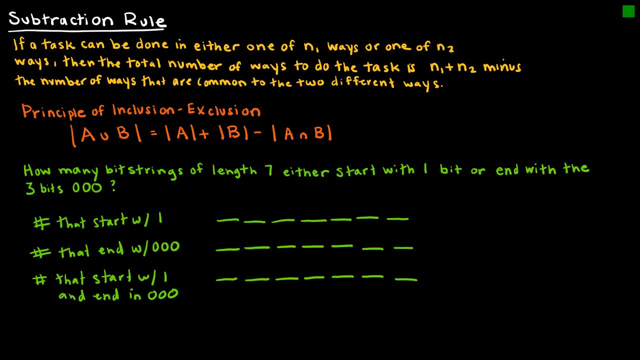 Then all I have to do is add the number of each of those choices to find the total number of choices. Now we have the subtraction rule And quite often you'll see this called the principle of inclusion exclusion, And we'll talk more in detail in this course, And then we'll talk in way more detail if 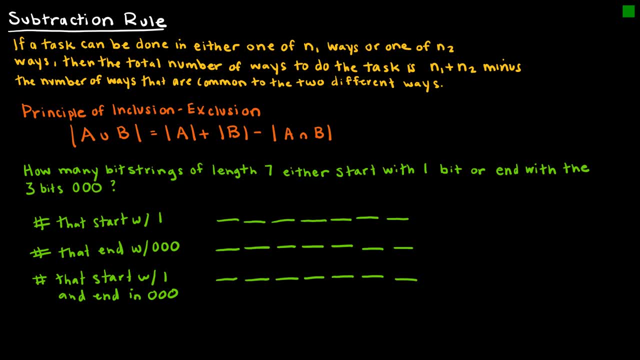 you continue on to combinatorics, But the subtraction rule basically says: if a task can be done in either one of n one ways or one of n two ways, then the total number of ways to do the task is n one plus n two, minus the number of ways that are common to the two different. 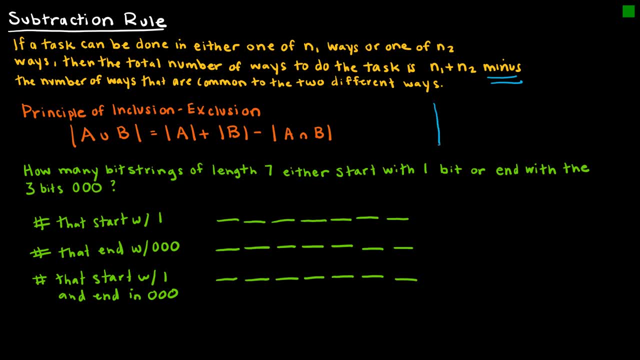 ways. So essentially, if you've taken any sort of statistics class, this is the rule that says: hey, if there's something here in the middle where those values are not disjoint, so there is an overlap of the number of ways in each set, then we have to subtract what's in the overlap, because 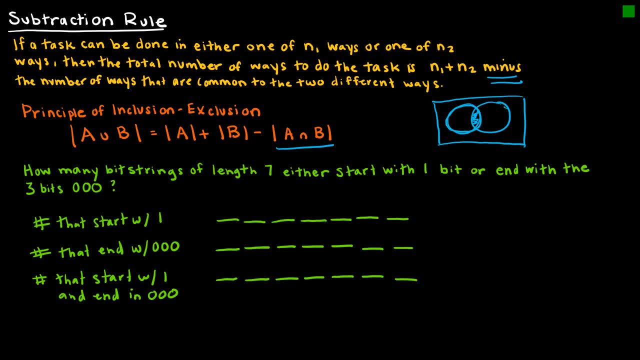 essentially it was counted in the first set and in the second set. So, for instance, how many bit strings? bit strings of length seven either start with one bit or end with three bits: 000.. So if I have the number that start with one, so I'm setting this value to be one, And then all of these is 123456. 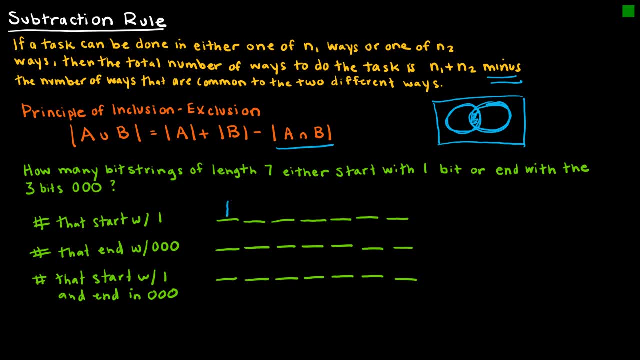 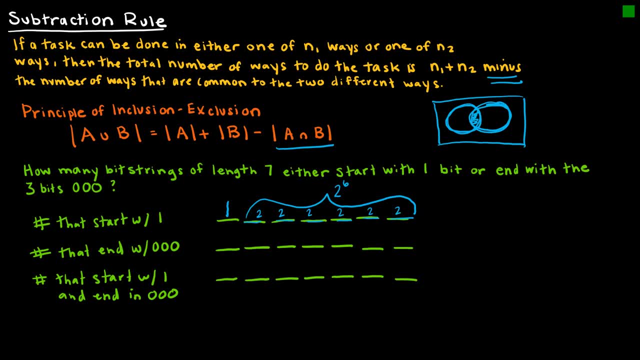 two here and two here, Remember, because a bit string is going to have values of zero or one. Now let's find the number that end with zero, zero, zero. So I'm setting this to be zero, setting this to be zero and setting this to be zero, And 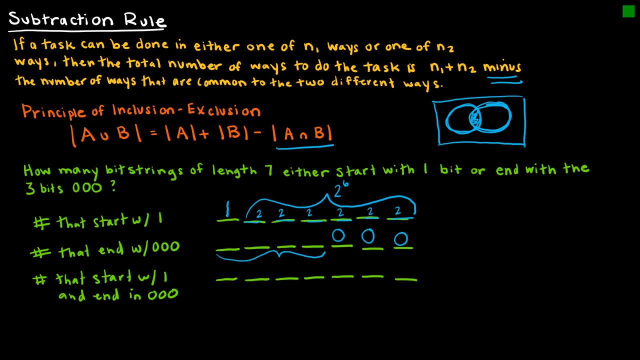 then again I've got any value that I want of the two, zero or one, so this could be one of two choices times one of two choices, times one of two choices times one of two choices. I should have put multiplication up there as well, And 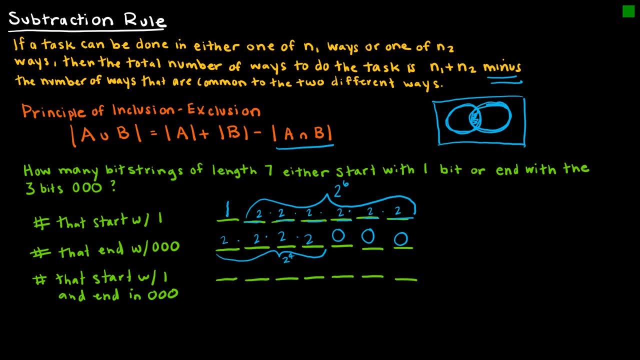 again, that's two to the fourth, So two to the fourth that end with zero, zero, zero. And now? so I've basically found this value, and now I'm going to- and I've already found this value- I need to find the overlap, The ones I counted both here. 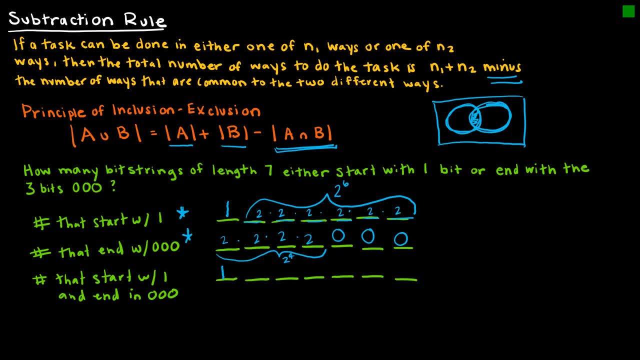 and here. So now I'm going to set the first value as one, The last three values as zeros, And these values can be anything I want them to be. So that's two times two times two, or two to the third. So my solution would be two to the. 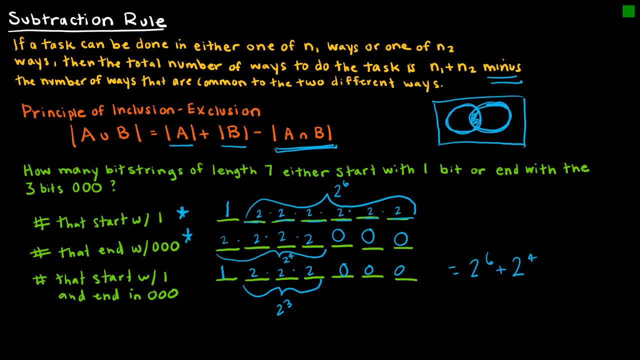 sixth, plus two to the fourth, minus two to the third. Now of course I could go through and determine that answer, Which is not going to be very difficult, Because two to the sixth is 64.. Two to the fourth is 16.. Two to the third is eight. So if I add 64 and 16, I get 80., 80 minus. 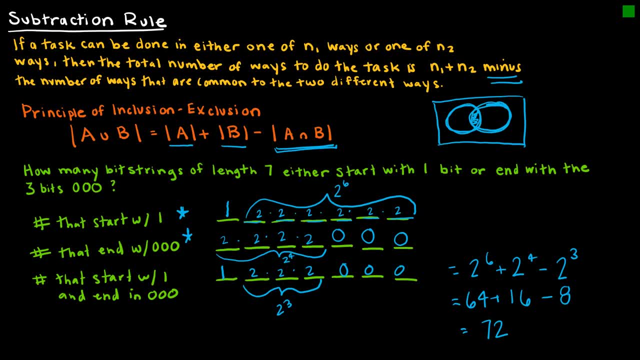 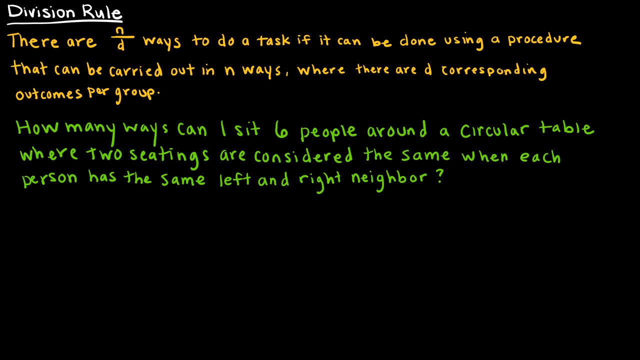 eight is 72. So there's 72 different ways Again, because there were eight that I counted in, both the numbers that start with one and and that end with zero, zero, zero. The last rule I would like to go over is the division rule, And the division rule essentially says there are N divided by 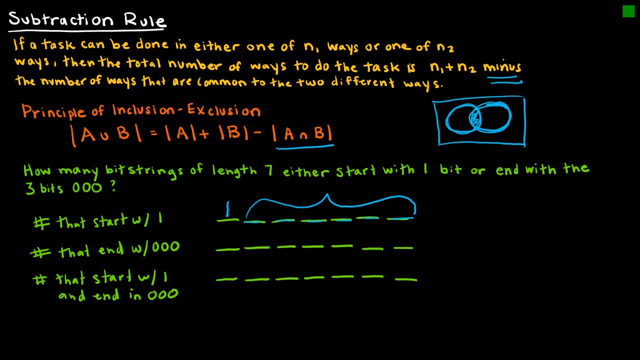 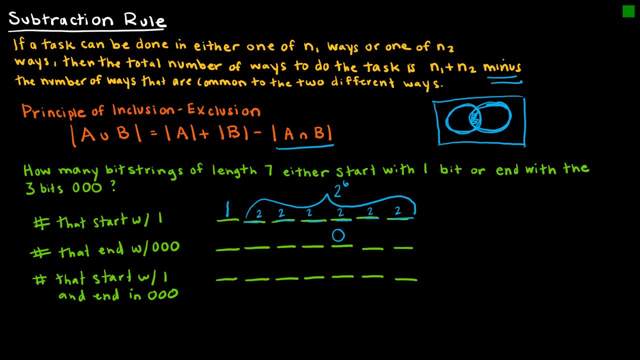 that end with 000.. So I'm setting this to be zero, setting this to be zero and setting this to be zero, And then again I've got any value that I want of the two, zero or one. So this could be one of two choices times one of two. 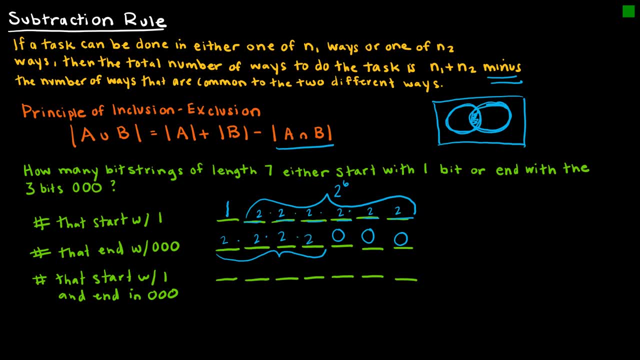 choices, times one of two choices, times one of two choices. I should have put multiplication up there as well. And again, that's two to the fourth. So two to the fourth that end with 000.. And now, so I've basically found this value, and now I'm going to, and I've already found this value, I 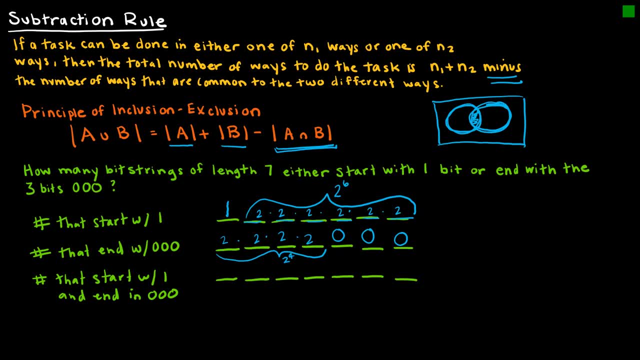 need to find the overlap, the ones I counted both here and here. So now I'm going to set the first value as one, the last three values as zeros, and these values can be anything I want them to be. So that's two times two times two or two to the third. So my solution would be two to the sixth. 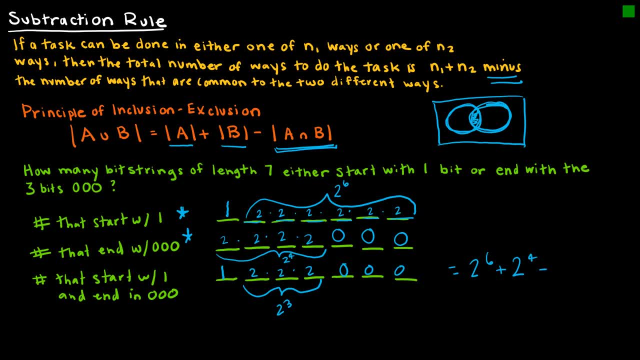 plus two to the fourth, minus two to the fourth. Now, of course I could go through and determine that answer, which is not going to be very difficult, Because two to the sixth is 64.. Two to the fourth is 16.. Two to the third is eight. So if I add 64 and 16,. 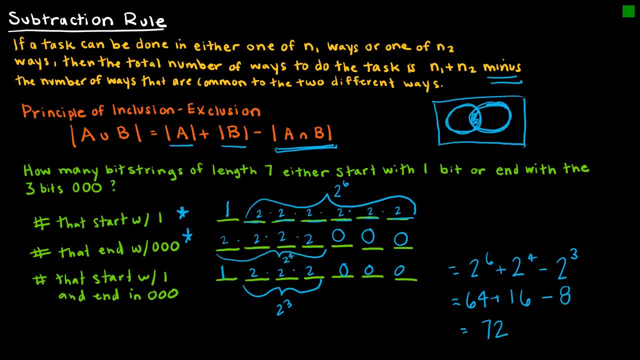 I get 80.. 80 minus eight is 72.. So there's 72 different ways to do this. So I'm going to put in the number of ways Again, because there were eight that I counted in, both the numbers that start with one and that end with 000. 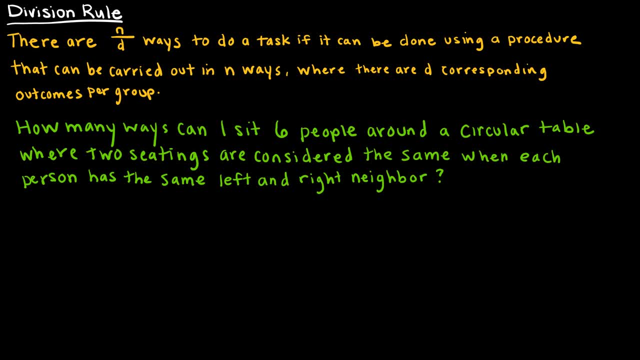 The last rule I would like to go over is the division rule, And the division rule essentially says there are n divided by d ways to do a task if it can be done using a procedure that can be carried out in n ways, and there are d corresponding outcomes per group. 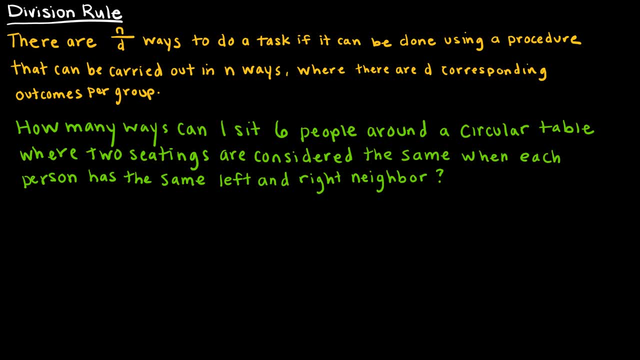 D ways to do a task, If it can be done using a procedure that can be carried out in N ways, And there are D corresponding outcomes per group. So that seems a little bit sketchy and maybe hard to understand. So let's take a look. 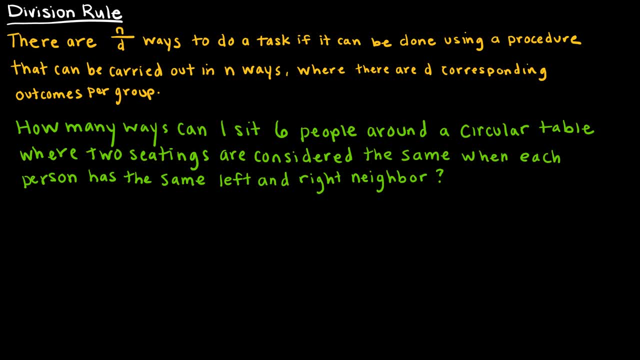 at an example and hopefully help us to understand. So I have a circular table And I'm going to split this table into six positions And I'm just going to arbitrarily call this position one, two, three, four, five and six. So it says: how many ways can I sit? eight people, I'm. 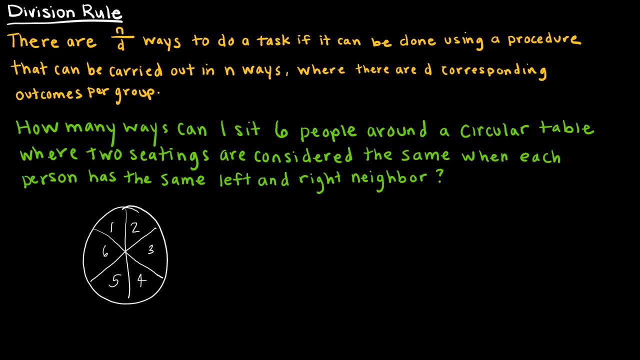 sorry, six people around a circular table where two seatings are considered the same when each person has the same left and right neighbor. So if I were just going to determine the number- and it was not considered the same when the person had the same left and right hand neighbor, I could very. 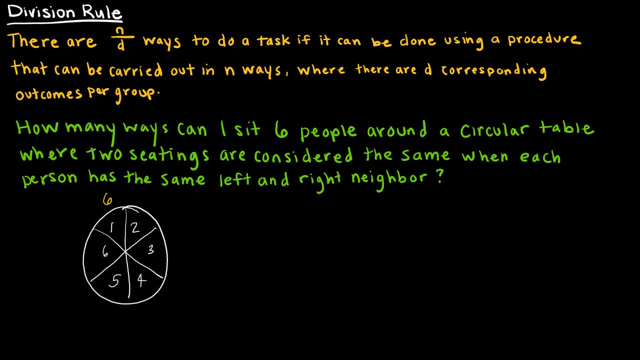 easily do this by saying there are six options for position one, because there are six people. Once I've sat one person in position 1, there are five people left for position 2 and four for position 3 and 3 and 2 and 1.. And so 6 times 4 to 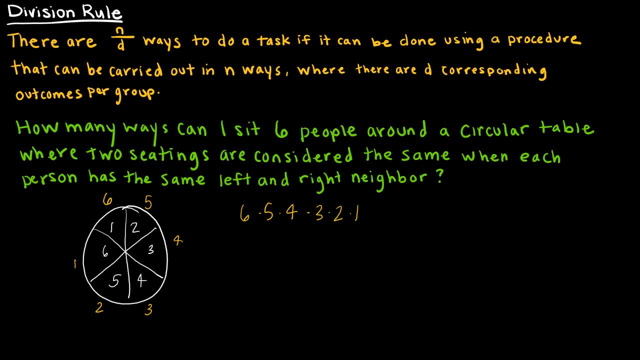 times six times five times, four times, three times two times one or six. factorial would be the total number of ways. Well, that's all well and good, But here's the problem. I'm going to erase my numbers here. Oh, and my circle, apparently. So let's say person A sat in position one. 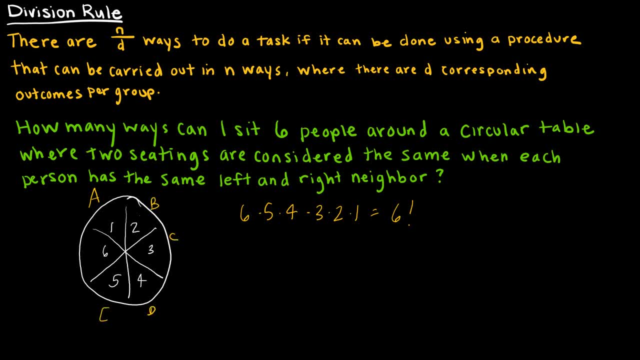 and then B, C, D, E and F, So Adam and Bob and Kurt and Doug and Eric and Frank. We get the idea What the what this is saying is. let's say instead: Adam sat here and Bob sat here. 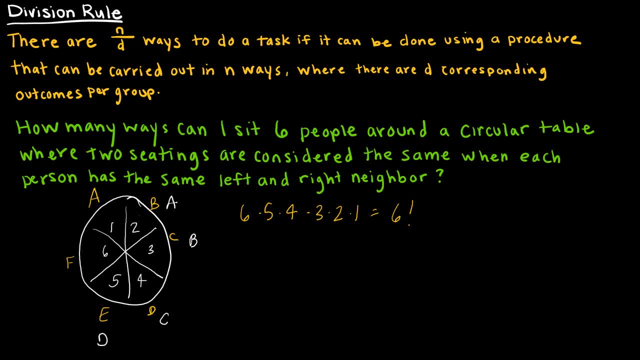 and I don't remember the names that I made up, So we'll just, you know, stick with my lettering system. So I have A, B, C, D, E, F. Notice, all I did was I took everyone and rotated them. 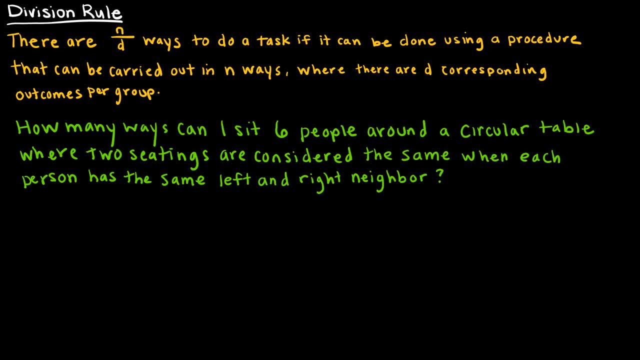 So that seems a little bit sketchy, Maybe hard to understand. So let's take a look at an example and hopefully help us to understand. So I have a circular table And I'm going to split this table into six positions And I'm just going to arbitrarily call this position one, two, three, four, five and six. 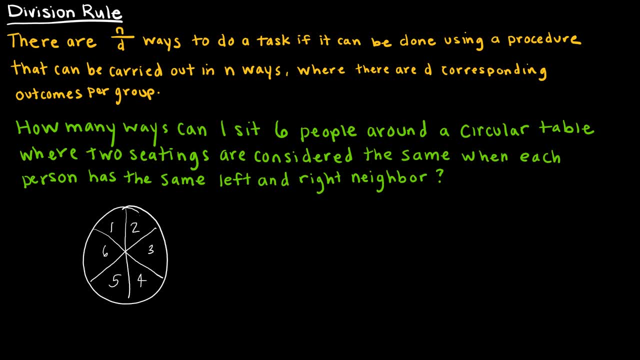 So it says: how many ways can I sit eight people, I'm sorry, six people- around a circular table where two seatings are considered the same when each person has the same left and right neighbor? So if I were just going to determine the number, and it was not considered the same when the person had the same left and right hand neighbor. 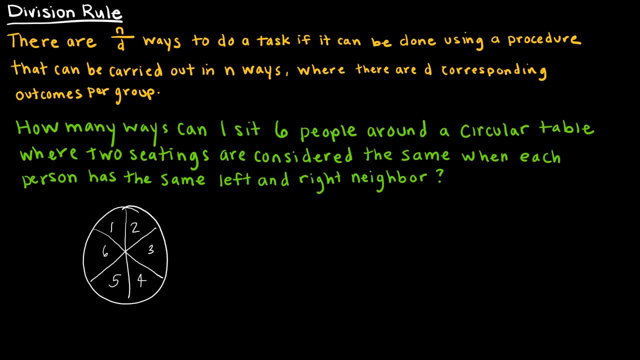 I could very easily do this by saying there are six options for position one, because there are six people. Once I've sat one person in position one, there are five people left for position two And for position two, there are five people left for position two. 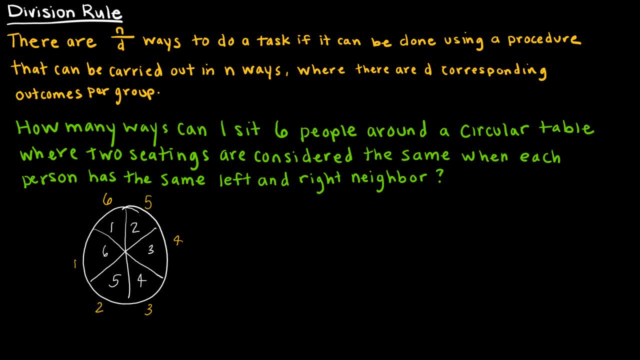 And for position three and three and two and one, And so six times four times six times five times four times three times two times one or six, factorial would be the total number of ways. Well, that's all well and good, But here's the problem. 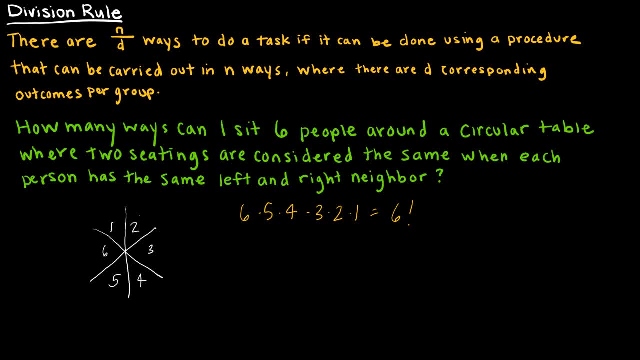 I'm going to erase my numbers here and my circle apparently. So let's say, person A sat in position one And then B, C, D, E and F, So Adam and Bob and Kurt and Doug and Eric and Frank. 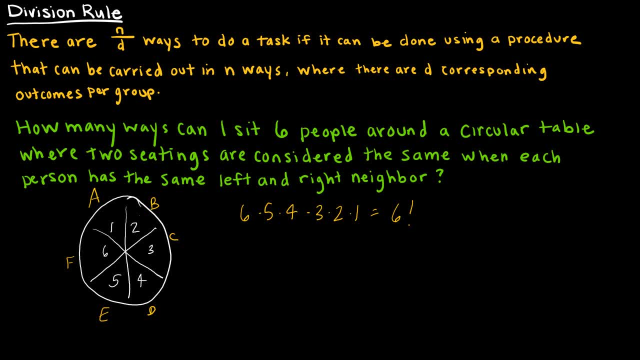 We get the idea What this is saying is. let's say instead: Adam sat here and Bob sat here, And I don't remember the names that I made up, So we'll just, you know, stick with my lettering system. So I have A, B, C, D, E, F. 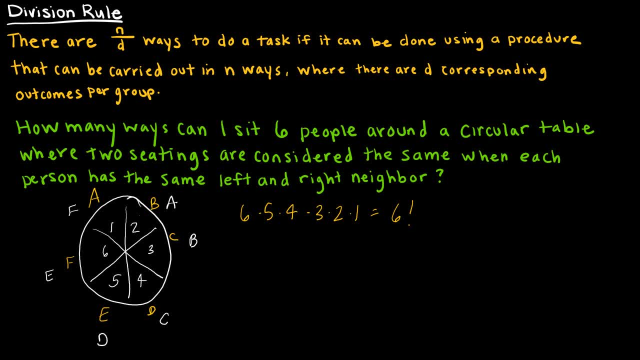 Notice. all I did was I took everyone and rotated them clockwise one position, And so these two seatings are considered the same. And again, if I shifted one more and said here's A and here's B and here's C and here's D and here's E and here's F,